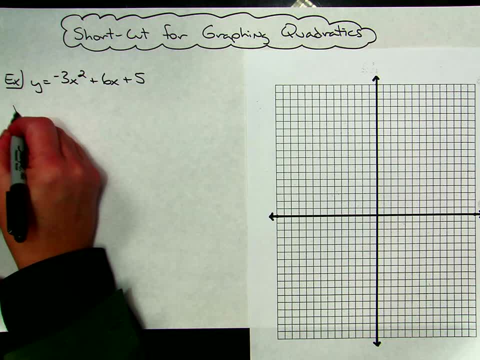 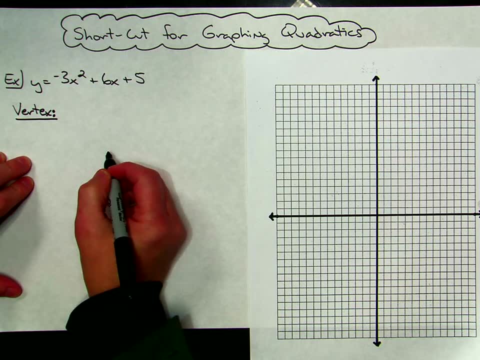 Okay, we are going to go through and find the vertex first. Alright, and that method will not change from you know, even if you're doing a standard xy table to graph this quadratic. Um, so we will use the formula negative b over 2a. 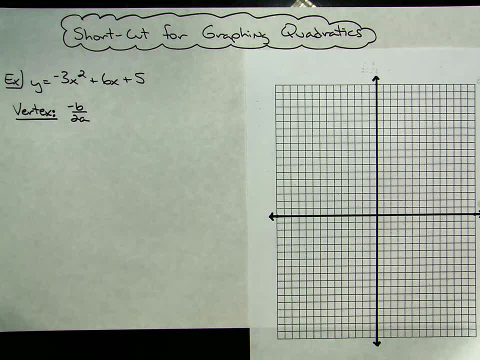 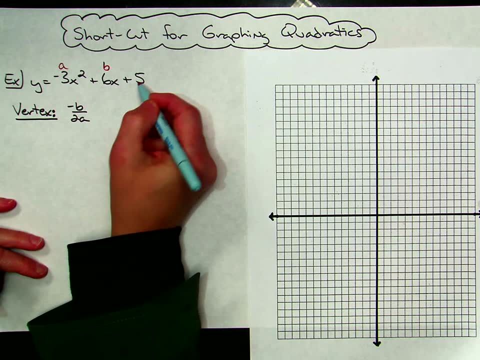 Alright, with each of these coefficients here, uh, representing a, b and c. So a would be the negative, 3, b would be the 6, and c would be the 5.. Okay, so we will take those coefficients and we will plug them into this formula. 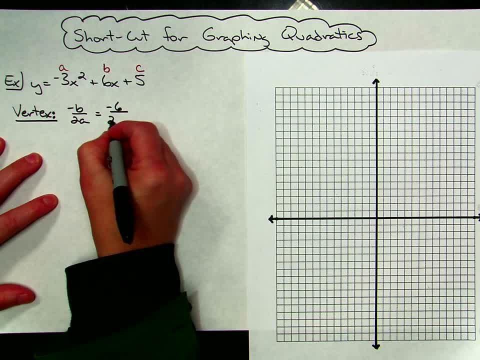 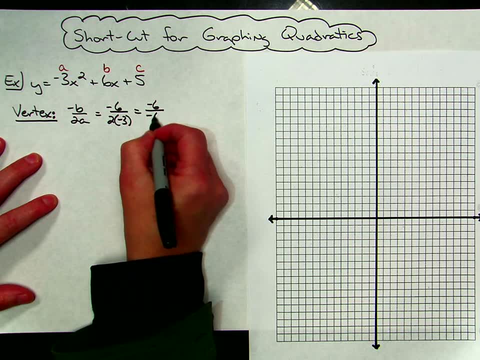 So a negative 6 over 2 times a negative 3.. Alright, simplifying, a negative 6 on top And a negative 6 on the bottom. Negative divided by negative is positive, And so I'm going to have a positive 1.. 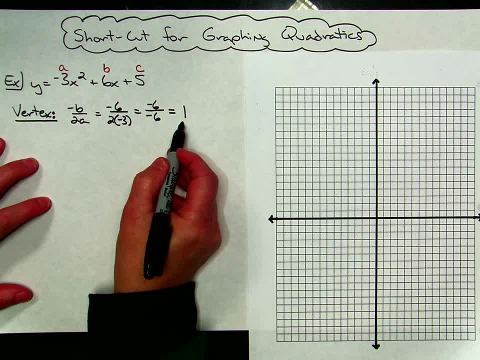 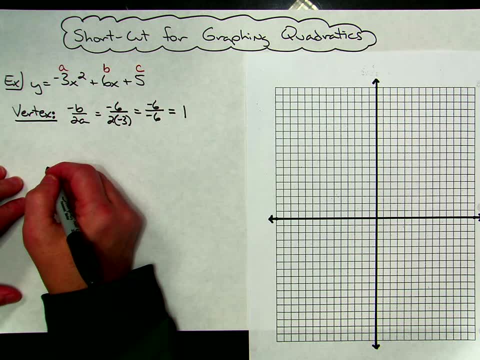 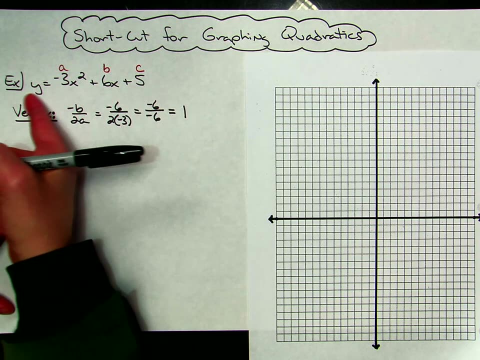 Okay, that is going to be the x coordinate of the vertex. Okay, so now I'm going to take that x coordinate of my vertex and plug it back into this function to find the y coordinate. Okay, so, in other words, if this was a function, say f of x, I would plug it back in here. 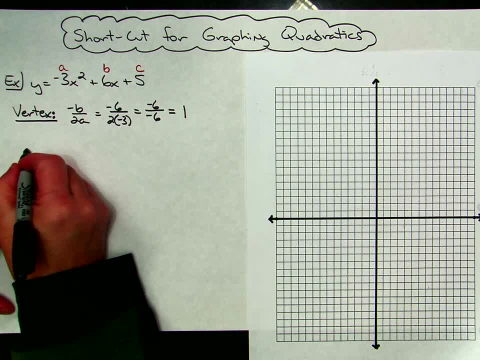 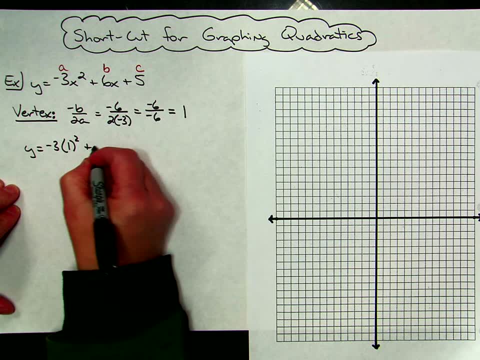 Or I could just go ahead and use the y notation: Y equals negative 3.. Y equals negative 3.. I'm going to plug the 1 back in: 1 squared plus 6, times 1, plus 5.. 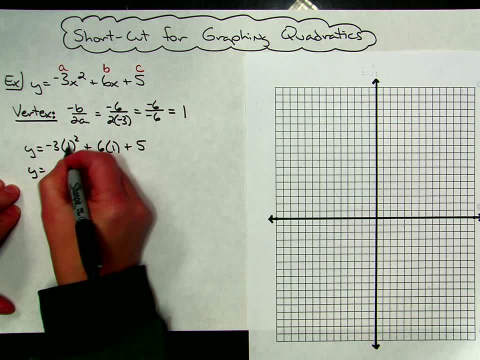 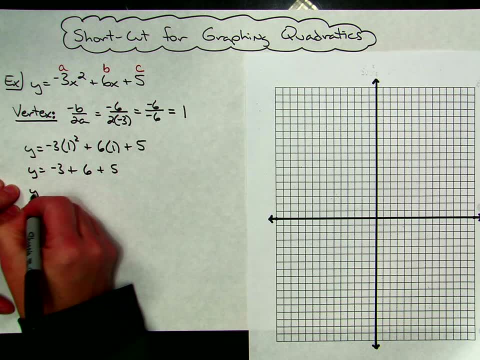 I'm going to work this out: 1 squared is 1, times negative 3.. 6 times 1 is 6, plus 5.. Okay, going left to right here, Uh, negative 3 plus 6 would give me a 3.. 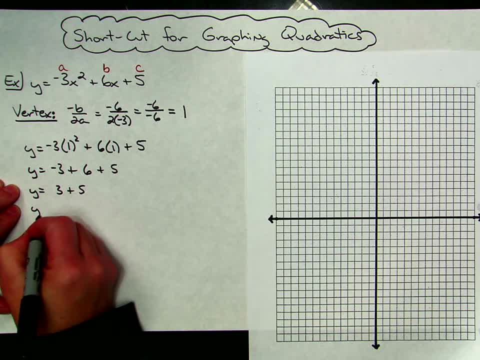 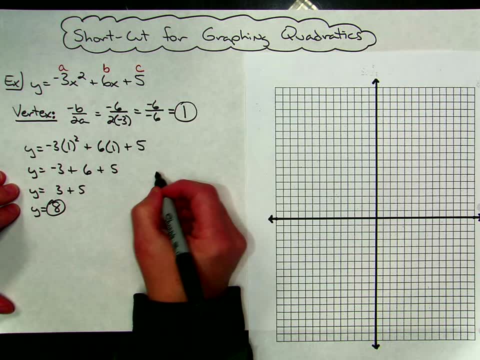 Plus 5 more, it's going to give me a y equals 8.. Okay, so from that I've got my x coordinate And my y coordinate, So my overall vertex is at 1, 8.. Okay, so there's my vertex. 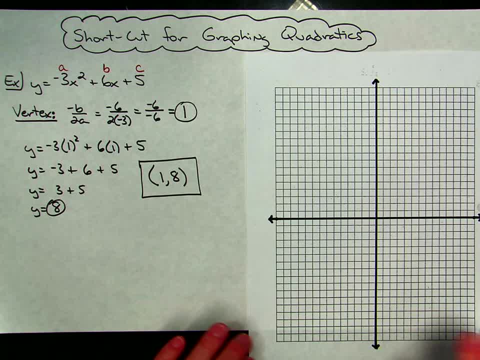 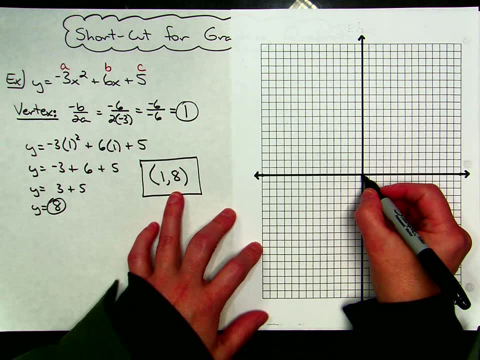 Alright, now that's going to be the first point that I plot on my graph paper here. Let's go ahead and move this up so it's a little bit more clear here. So I'm going to put a point at 1, 8.. 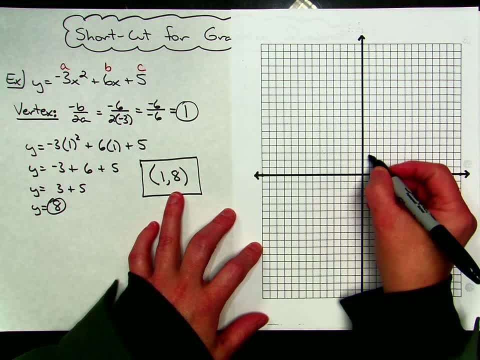 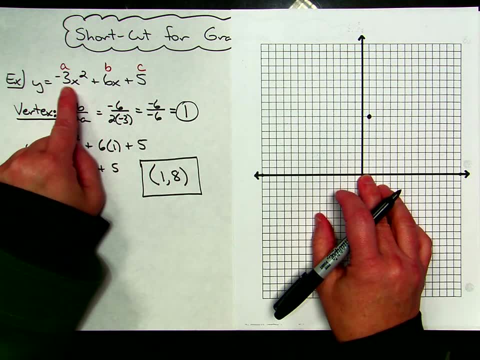 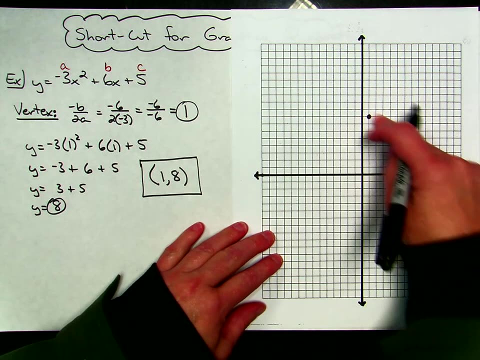 So over 1 and up 8.. It's right there, Okay. Now, looking at this quadratic, And it has a leading negative 3a coefficient. I know that this quadratic is going to be upside down, Okay. So I know that right off the bat. 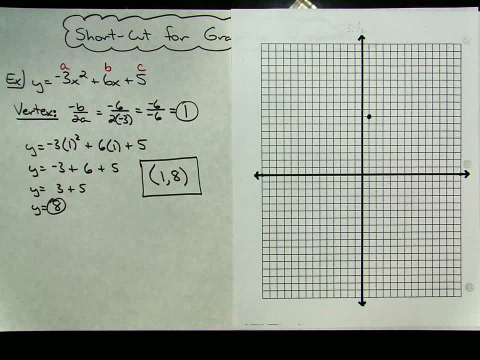 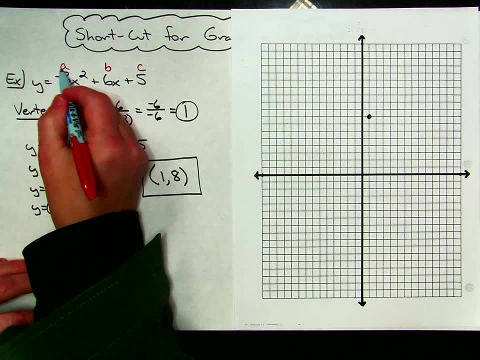 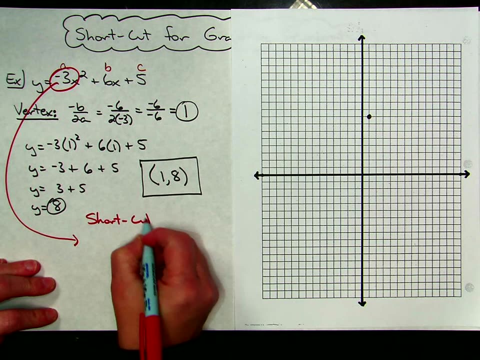 What I'm going to do is I'm going to take my a coefficient. Alright, so my a coefficient is negative 3.. Okay, This is for my shortcut. I'm going to take that a coefficient And I'm going to write it down 3 times. 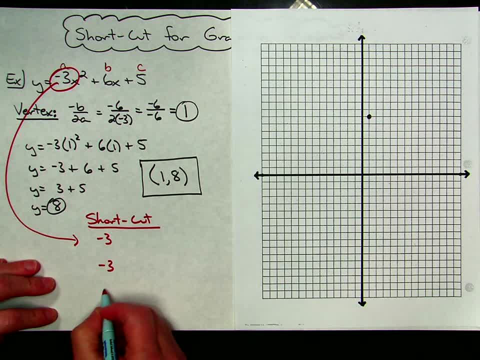 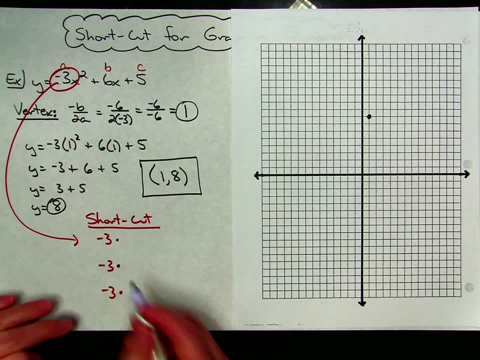 So negative 3, negative 3, negative 3.. Okay, Now what I'm going to do is the magic numbers always are going to be 1,, 3, 5.. So 1,, 3, 5. I'm going to multiply my a coefficient by 1,, 3, 5 every time. 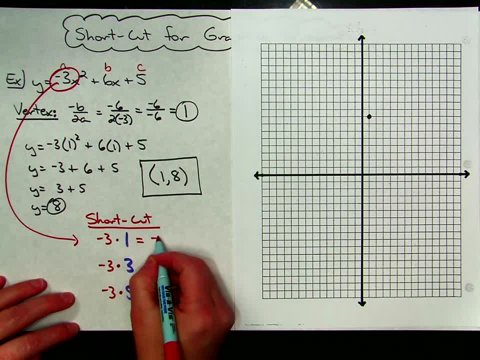 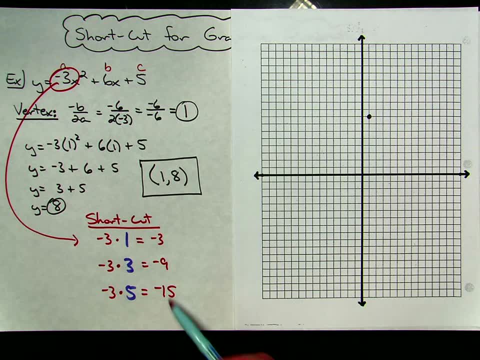 Okay, That's going to give me a negative 3.. That will give me a negative 9.. And that will give me a negative 15.. Alright, Now these numbers are going to be our shortcut. Okay, We are going to always move left to right 1 from our vertex. 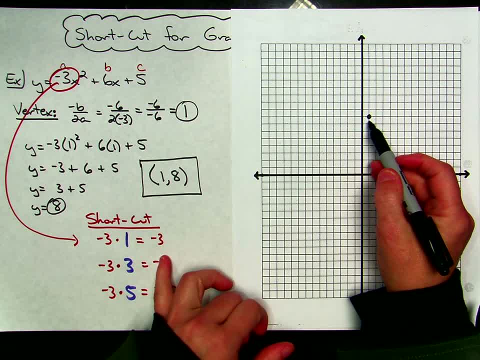 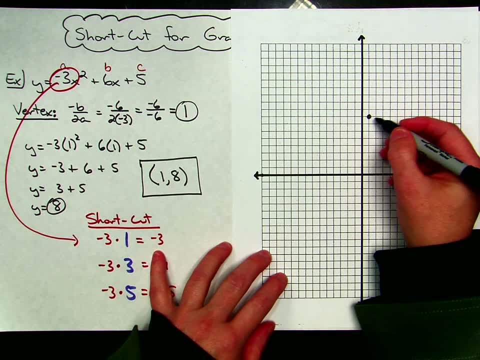 And then, in this case, since it's an upside down parabola, I'm going to be going down 3 and then down 9, and then down 15.. So I'm going to start the vertex, I'm going to go to the right- 1- and then down 3.. 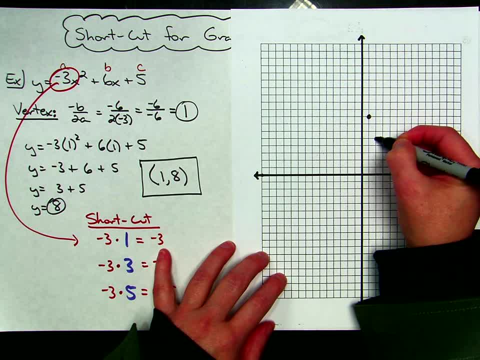 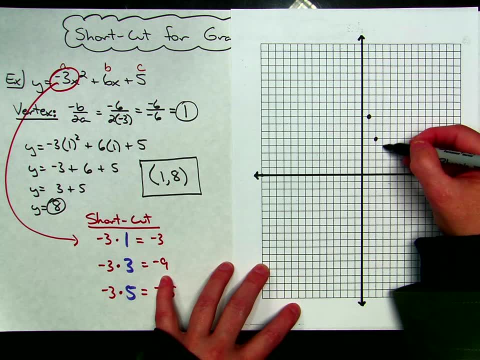 1,, 2,, 3. And I'm going to put a dot there, Alright, Then from that dot I will go 1 to the right again and then down 9. 9.. And that will be another dot on my parabola. 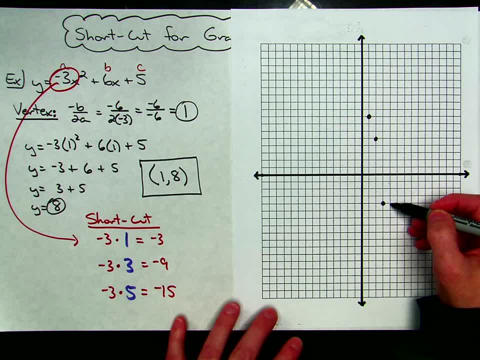 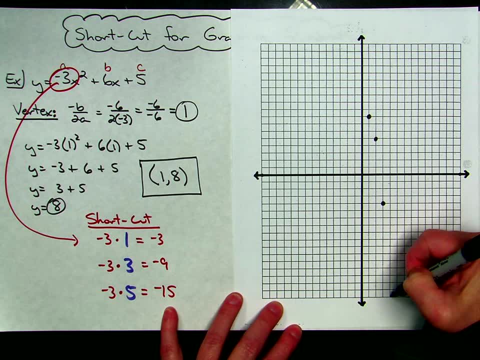 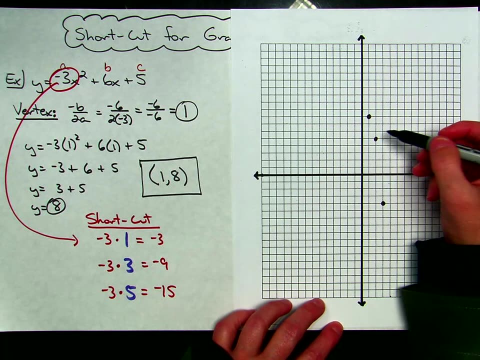 Now I'm going to go 1 to the right and down 15. And 13.. It's going to go off my graph paper, so I'm not going to worry about that one. Alright, Now, considering that all parabolas and quadratics are symmetrical, I know that there will be a corresponding point if I would go to the left one. 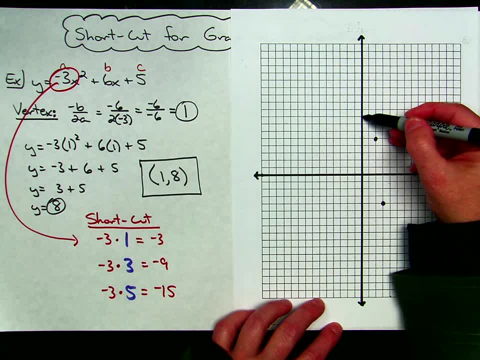 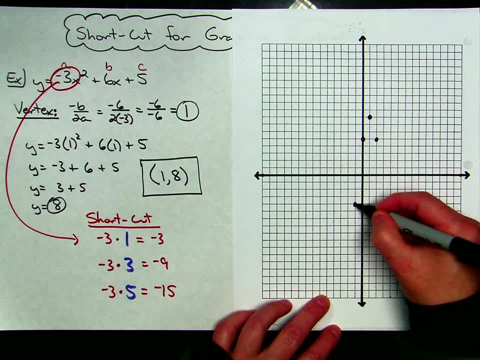 So if I go to the left one, I can come down to where that first dot was, And if I go to the left one more, then I can come down to the next dot. Alright, This is quicker than doing the traditional XY table. 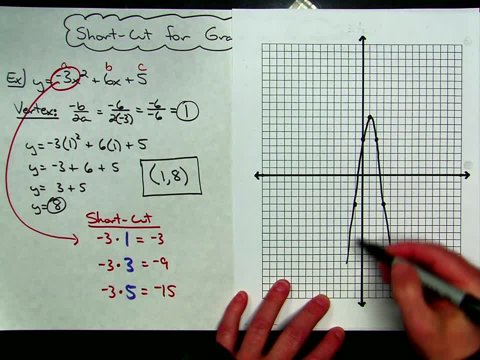 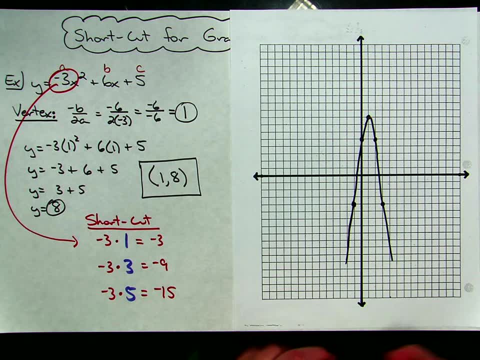 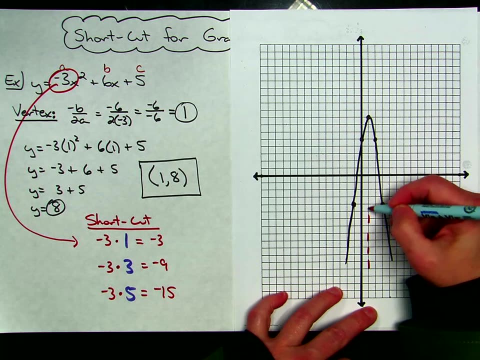 Alright And will work every time. and it doesn't make any difference whether the quadratic is upside down or right side up. Okay, Depending on your teacher. Some teachers might want you to go ahead and put in the axis of symmetry, Showing that that clearly is the center. 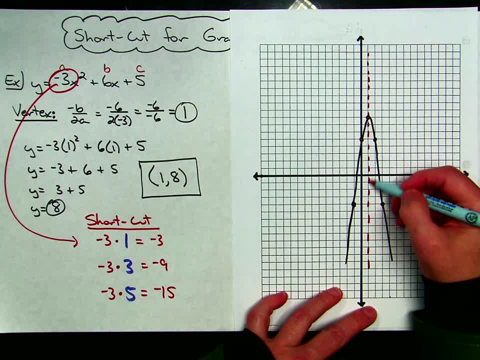 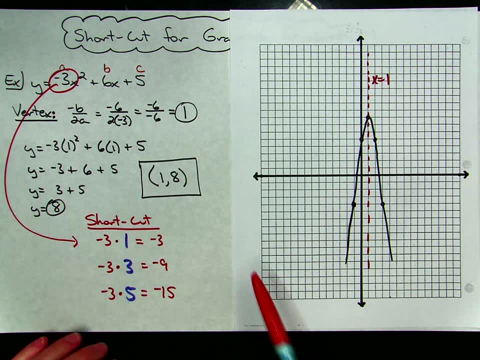 And some even want you to label that The axis of symmetry. here would be: an X equals 1. for that, Alright. So shortcut graphing for when the parabola, or quadratic, is in standard form: Alright. Now let's run another example. 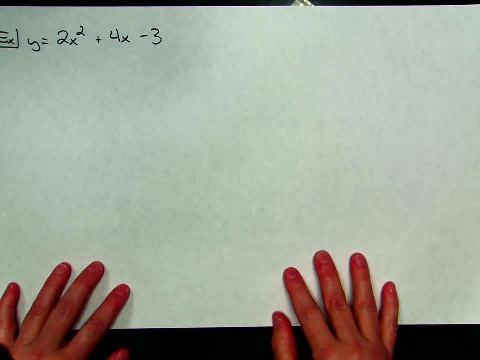 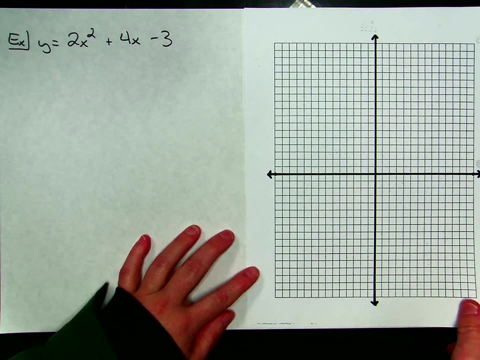 In this one, we will run one that is an upright parabola, Just to show you that the shortcut works for both An upside down and a right side up parabola. Okay, Now finding your vertex again always remains the same, Okay. 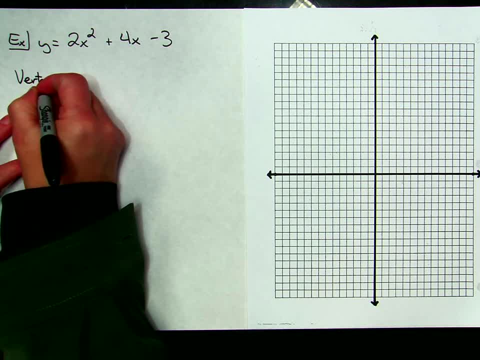 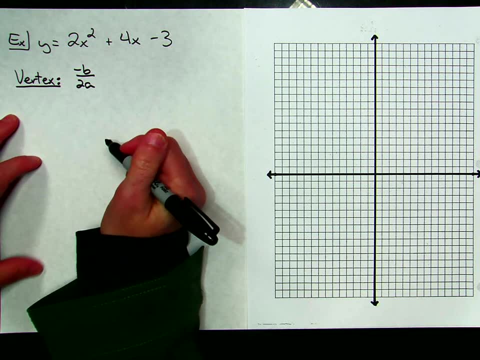 So my vertex: I want to find the X coordinate first, So I'm going to use the formula negative B over 2A. That's a formula that you're just going to have to memorize for finding your X coordinate of your vertex. Okay, 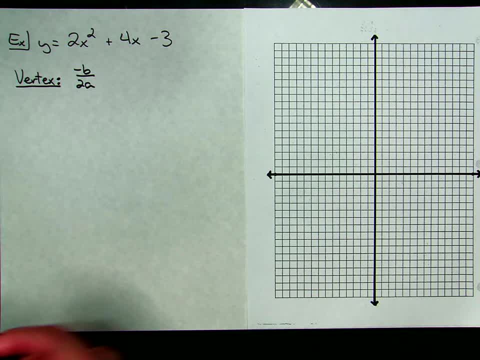 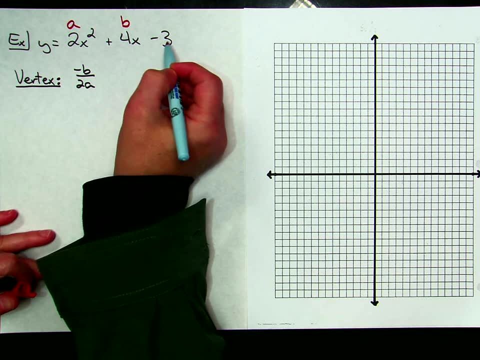 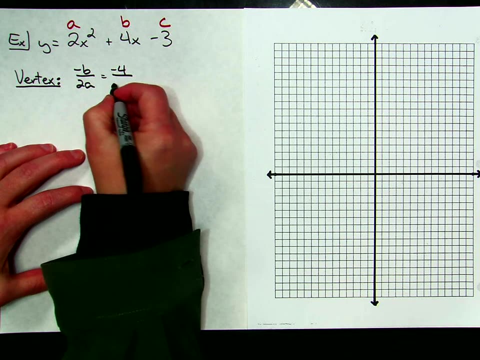 Again, if you need to label the A, B and C in your quadratic, The 2 would be A, The 4 would be B And the negative 3 there would be my C. Alright For this formula. we would then have a negative 4 over a 2 times 2.. 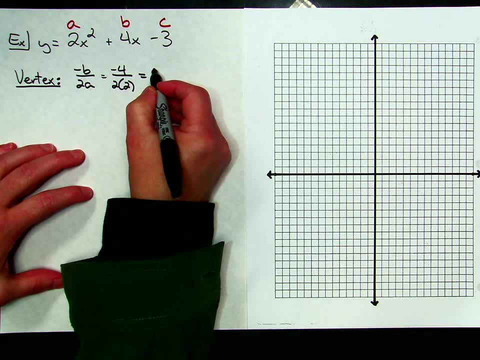 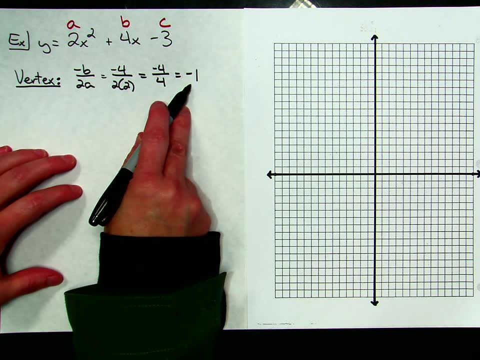 Simplifying there, Negative 4 over 2 times 2 would give me a 4. And that's going to give me a negative 1.. So the X coordinate of my vertex is going to be a negative 1. Then I'm going to take that negative 1.. 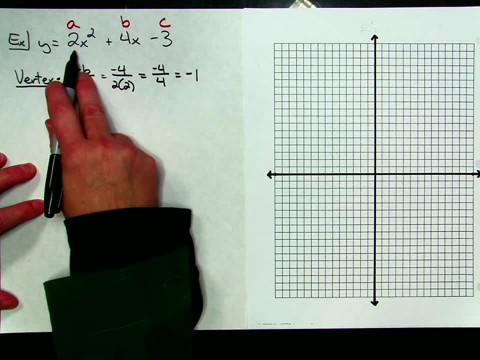 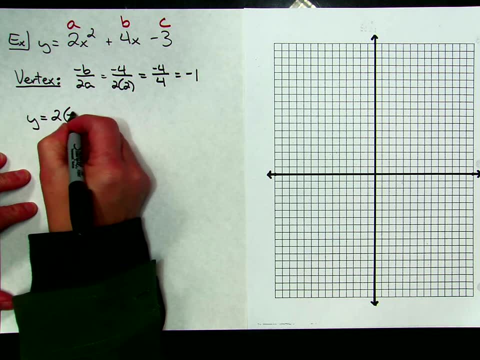 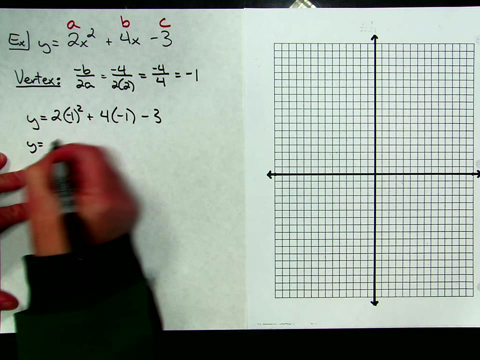 I'm going to plug it back into my quadratic To find my Y. So Y equals 2 times a negative 1 squared, Plus 4 times a negative 1 minus 3.. Okay, Simplifying Negative 1 squared would be 1 times 2 is going to give me a 2.. 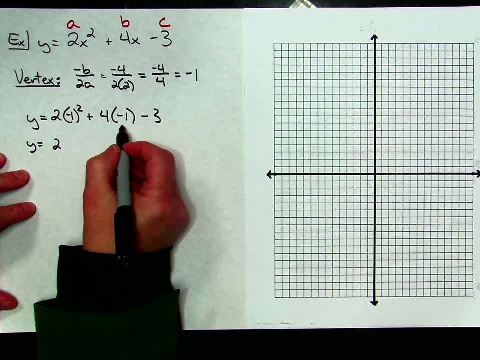 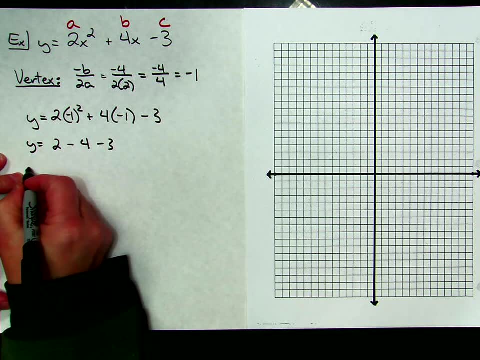 Negative 4 or 4 times a negative 1 will give me a negative 4.. So minus 4.. And then the minus 3.. Going left to right here: 2 minus 4.. 2 minus 4 will give me a negative 2.. 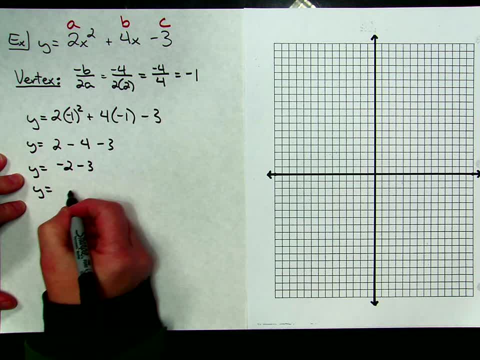 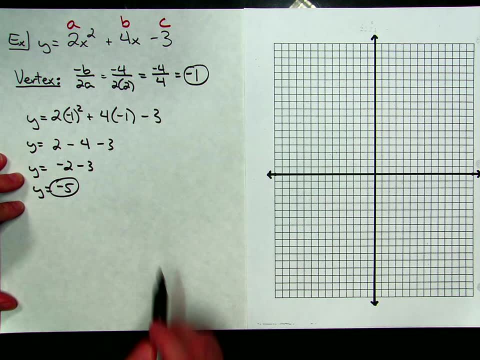 Minus 3.. Final answer: Y here is going to be a negative 5.. So there's my Y coordinate And there's my X coordinate of my vertex. So I can write the ordered pair as negative 1, negative 5.. 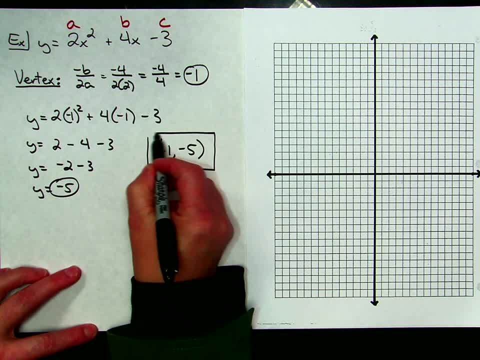 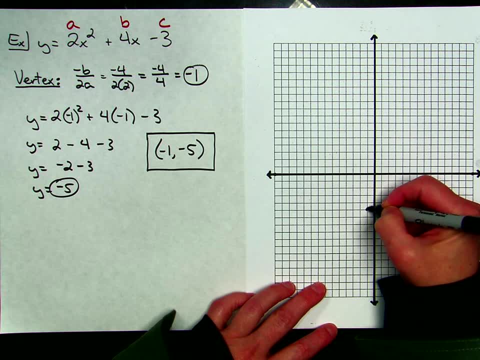 And that's going to be my vertex to my quadratic. So I'm going to come over And go to the left one and down 5. And that will be the vertex of my quadratic. And I know by looking at my A coefficient: it's a positive. 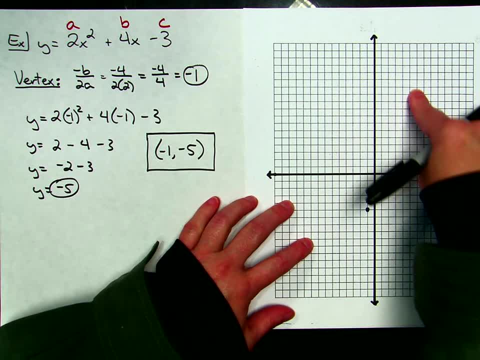 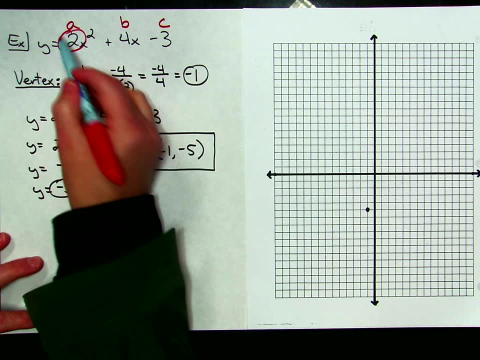 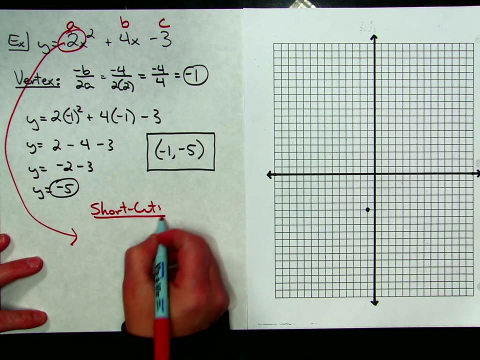 So I know this is going to be an upright parabola. Okay, Now I'm going to go through And I'm going to calculate my shortcut. I'm going to use the A coefficient every time for my shortcut. So I'm going to write 2, 2, 2.. 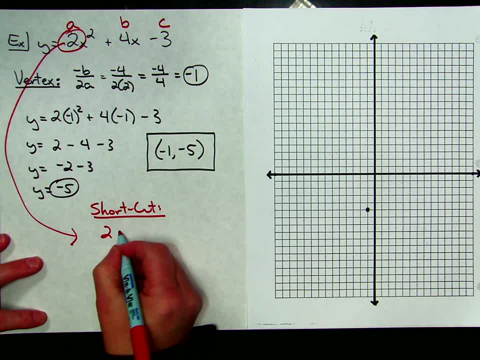 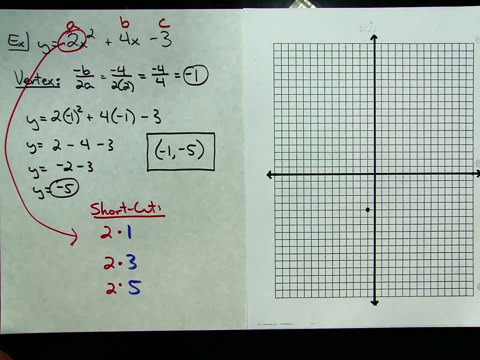 I'm going to do it 3 times, Alright, And then every time I'm always going to multiply by a 1,, 3,, 5.. Those are the magic numbers, And when I multiply that out 2 times, 1 is 2.. 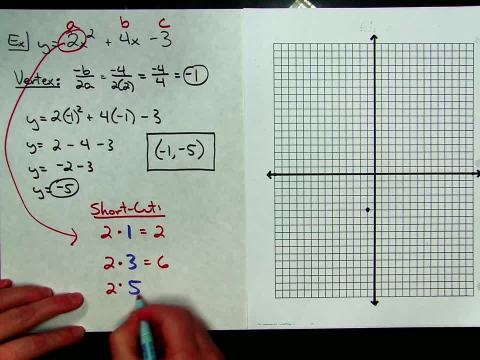 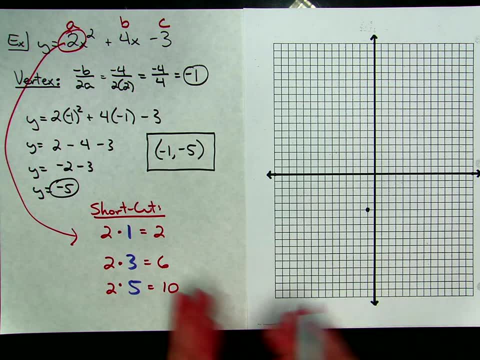 2 times 3 is 6.. 2 times 5 is 10.. Alright, So these are the numbers that I will be going up. Alright, I always move 1 to the right and to the left, And that's how many I will move up. 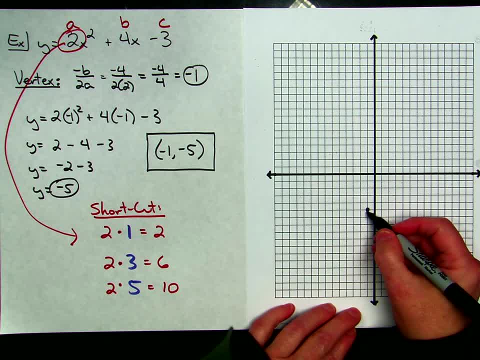 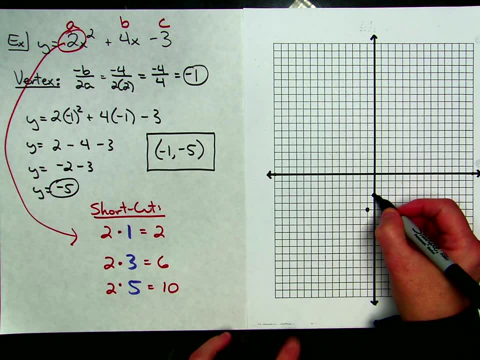 Alright. So, starting at my vertex, I'm going to go 1 to the right And then up 2. And put it up. I'm going to start from that point right there. I'm going to go 1 over And then up 6.. 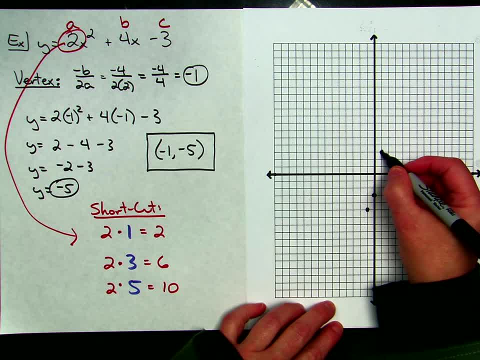 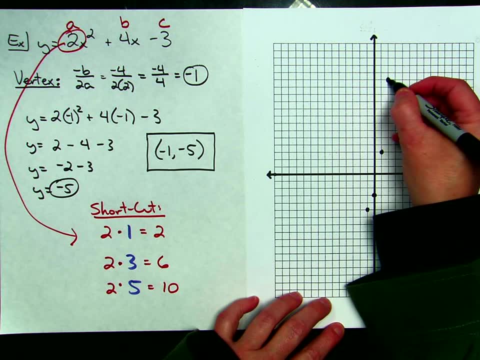 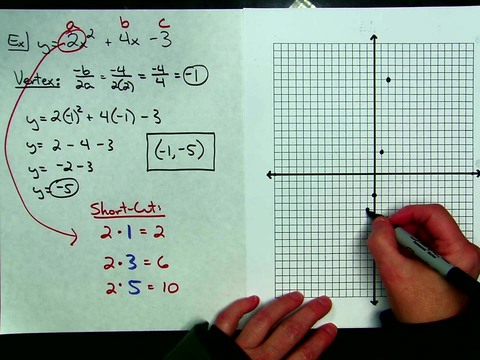 And put a dot. I will go 1 to the right And then up 10. And there's the 3 dots on my parabola. Now Parabola is symmetrical around that axis of symmetry, So I can do the exact same thing going to the left. 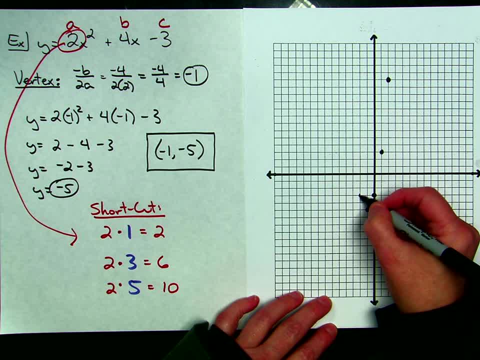 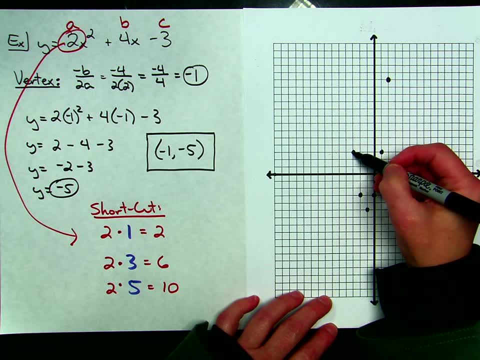 So, going to the left, 1. I can go up 2.- And it should be symmetrical- across from that other point, I can go over 1. And up to the next point, And then I can go over 1. And up to the last point. 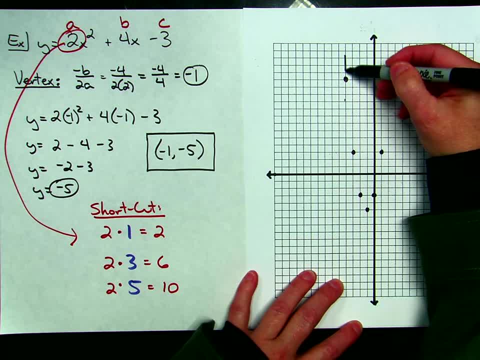 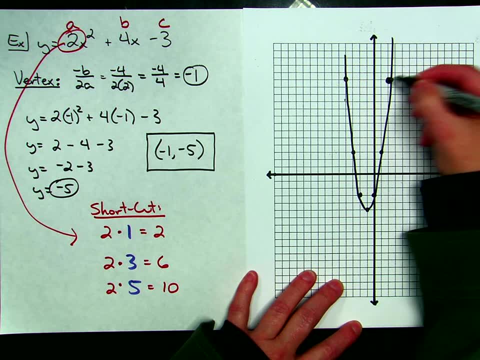 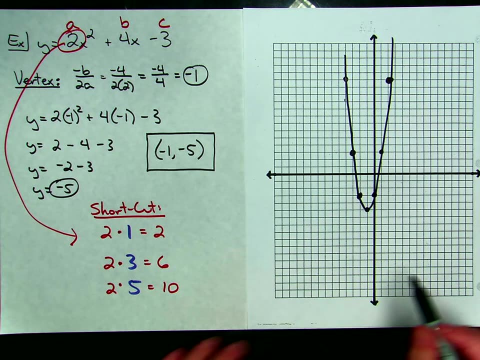 Alright, Just an alternative shortcut to graphing your parabola. And actually, Oops, Didn't kind of make it through that one Kind of definitely faster than attempting to make the XY table. Okay, But the shortcut involves remembering 1,, 3,, 5..